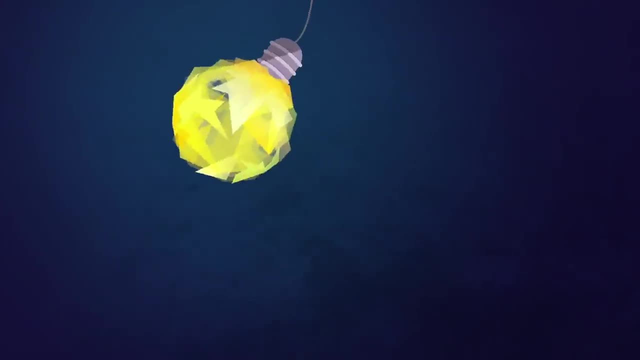 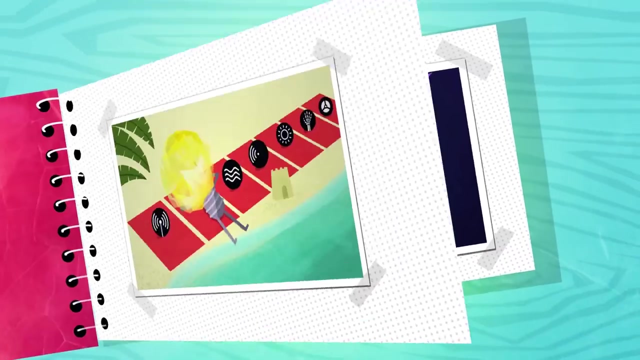 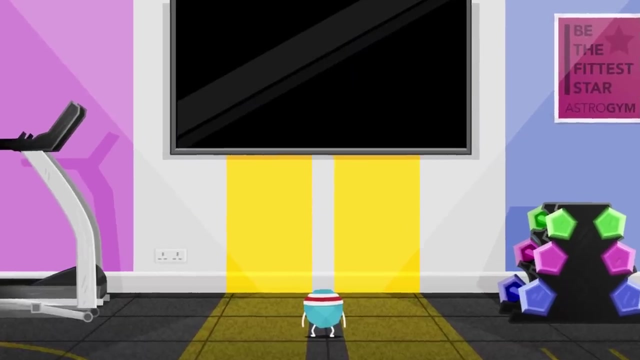 Light is a strange thing. It isn't just what we can see. Light can be broken up into different types and we call the whole family the electromagnetic spectrum. So even when it's dark, light is still all around us. Light can be created by making an electron oscillate. This creates 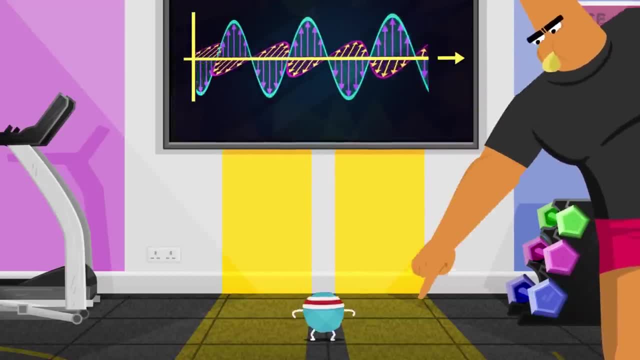 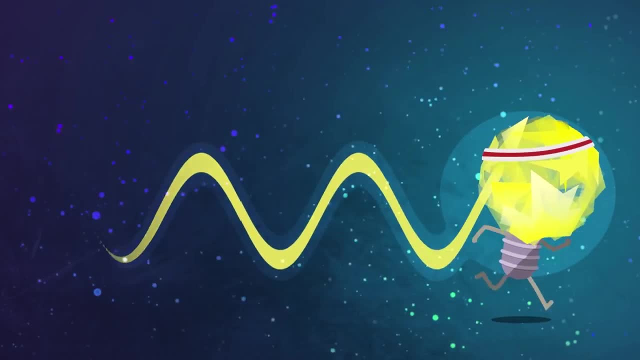 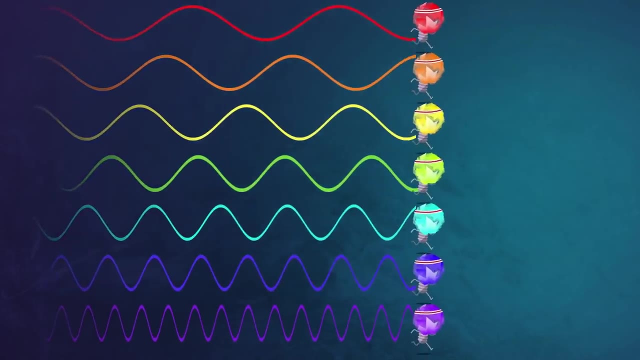 an oscillating magnetic field and an oscillating electric field, which we call an electromagnetic wave or light. We often represent light as a wave. Just like water waves, light has a wavelength, a frequency and a speed. The different colours of optical light have different wavelengths. 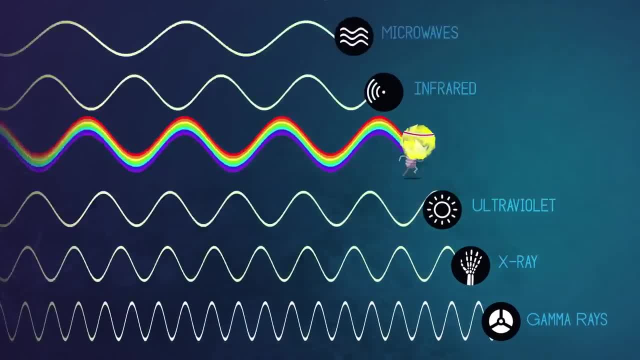 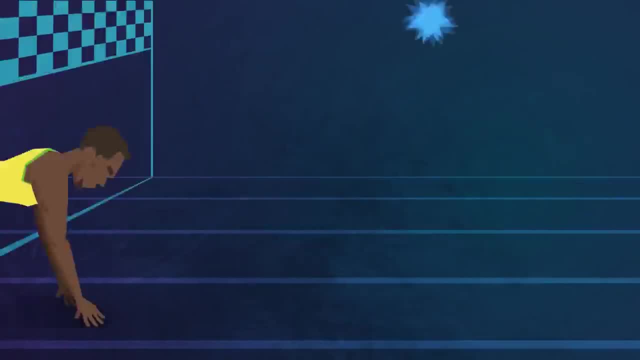 and so does the rest of the electromagnetic spectrum. Gamma rays are the most energetic, whereas radio waves have the least energy. Even so, light is the fastest thing in the universe. In a vacuum, all light waves, even radio waves, travel at an incredible speed. 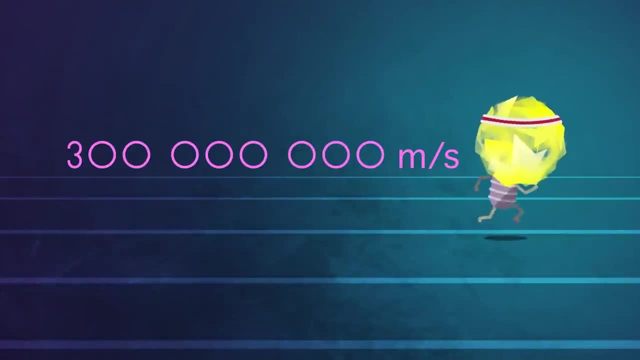 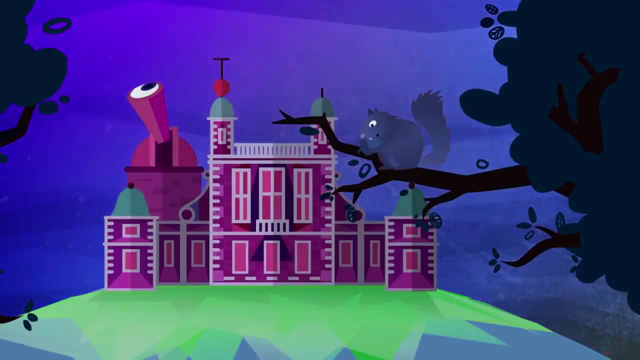 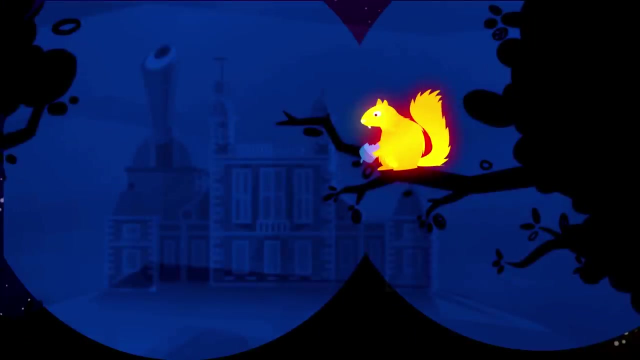 of 300 metres per second. The Royal Observatory is overrun with squirrels. They're hard to miss during the day, because they reflect visible light from the sun, but at night it's more difficult. However, they do emit infrared light and if our eyes could detect it, we would be able to see them in. 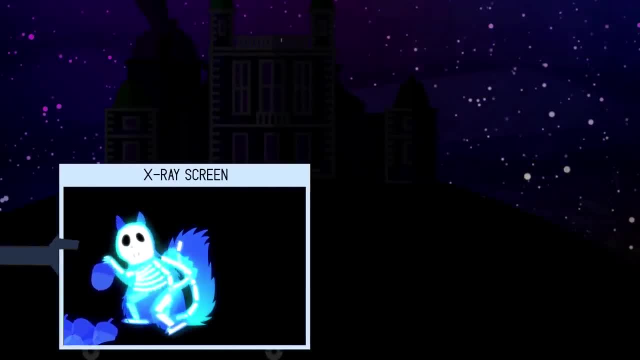 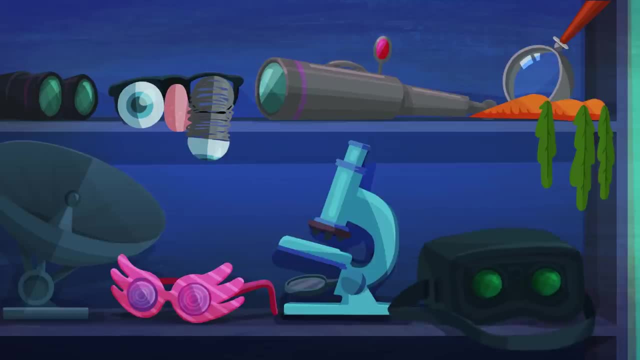 the dark. If we pass high-energy X-rays through them, the squirrels look very different. Humankind has invented lots of different instruments to show us what our eyes can see, Like our Great Equatorial Telescope, which captures huge amounts of light and allows 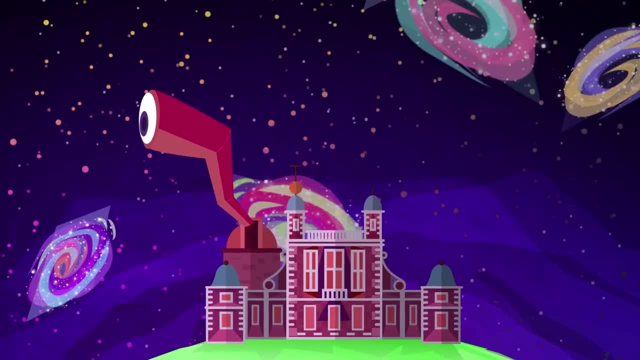 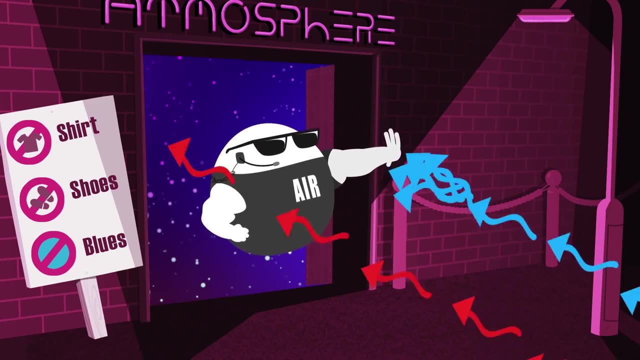 us to see objects that are tens of millions, of trillions of kilometres away. We can see matter interact with light and change it. The gases in the Earth's atmosphere scatter blue wavelengths of sunlight, giving us blue skies during the day and red skies at sunrise. 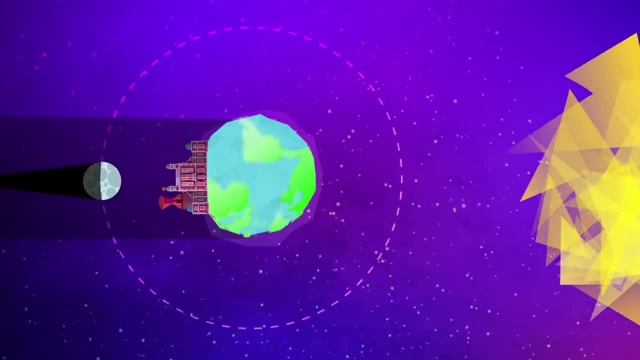 and sunset. We can watch sunlight reflect off planets and the moon During a lunar eclipse. red sunlight changes the light. We can also see light reflected off of planets and the moon During a lunar eclipse. red sunlight changes light. We can also see light reflected off of planets and the moon During a lunar eclipse. 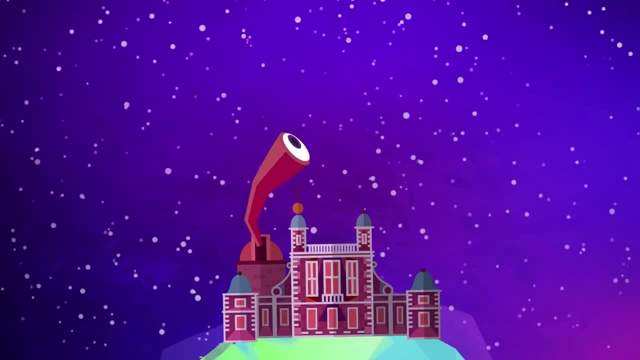 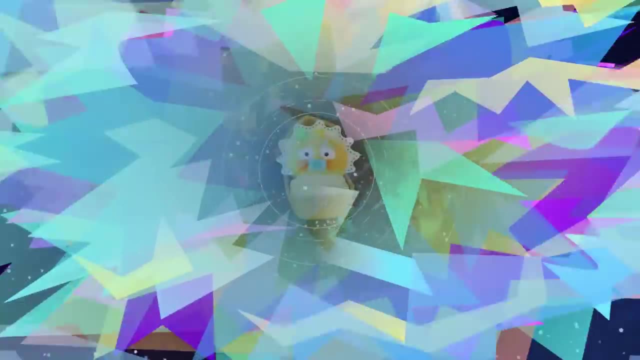 light is reflected off of planets and the moon. There is no special direction as it passes through the Earth's atmosphere and reaches the moon, And although visible light from stars can be absorbed by dust, in space we can detect the infrared light which gets 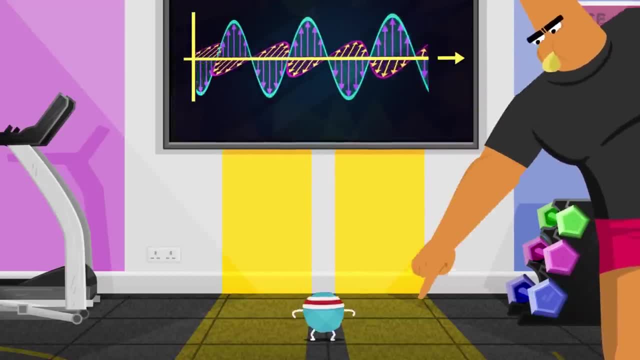 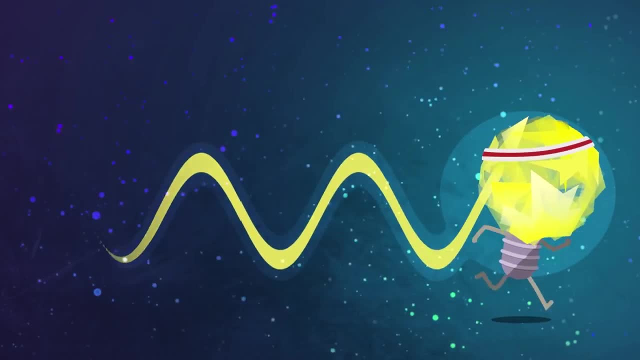 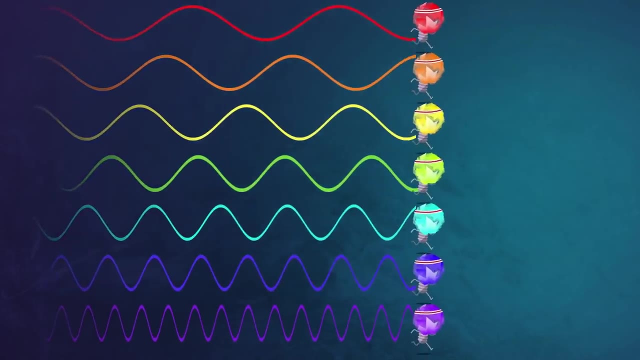 an oscillating magnetic field and an oscillating electric field, which we call an electromagnetic wave or light. We often represent light as a wave. Just like water waves, light has a wavelength, a frequency and a speed. The different colours of optical light have different wavelengths. 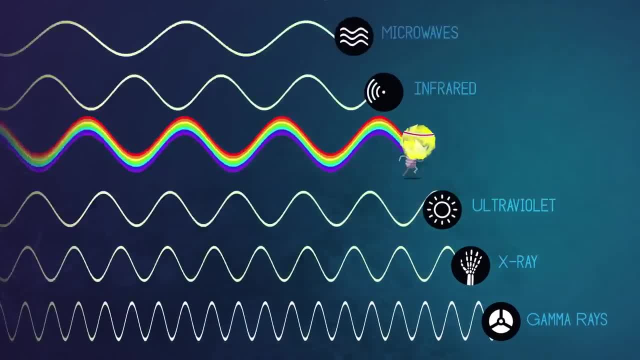 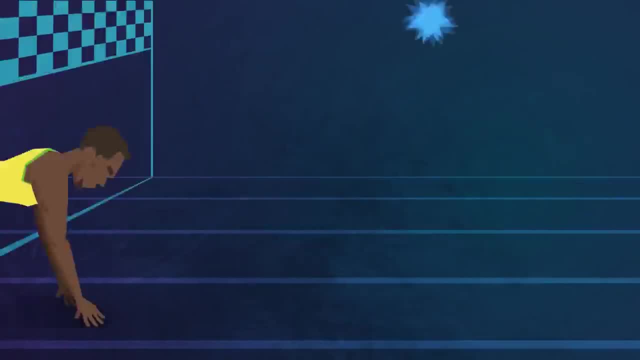 and so does the rest of the electromagnetic spectrum. Gamma rays are the most energetic, whereas radio waves have the least energy. Even so, light is the fastest thing in the universe. In a vacuum, all light waves, even radio waves, travel at an incredible speed. 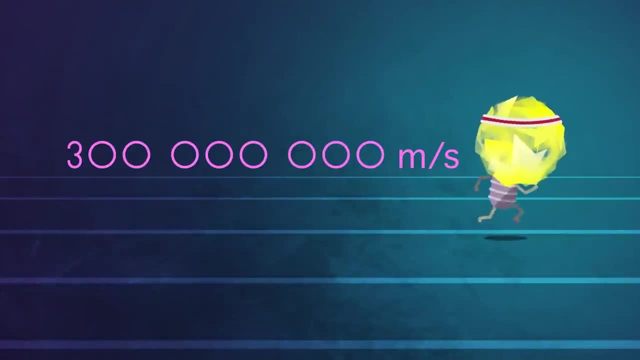 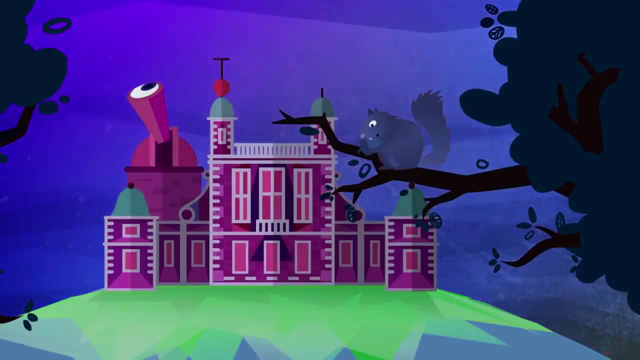 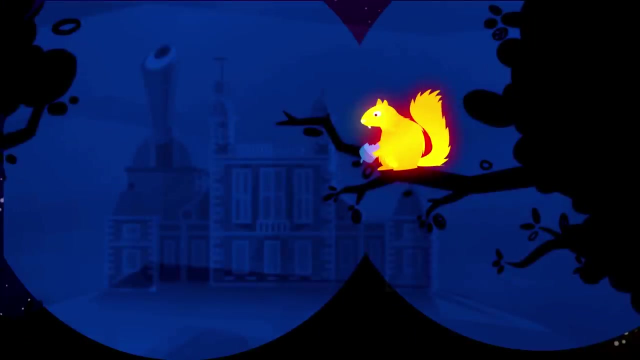 of 300 metres per second. The Royal Observatory is overrun with squirrels. They're hard to miss during the day, because they reflect visible light from the sun, but at night it's more difficult. However, they do emit infrared light and if our eyes could detect it, we would be able to see them in. 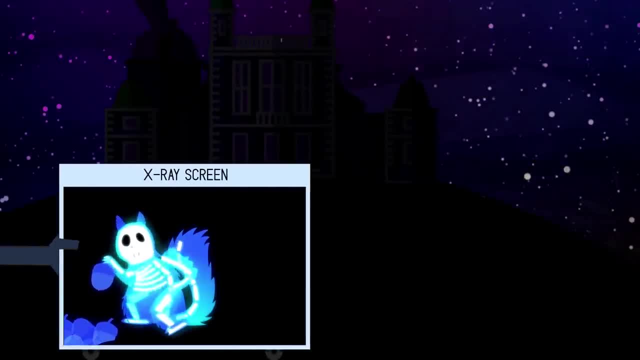 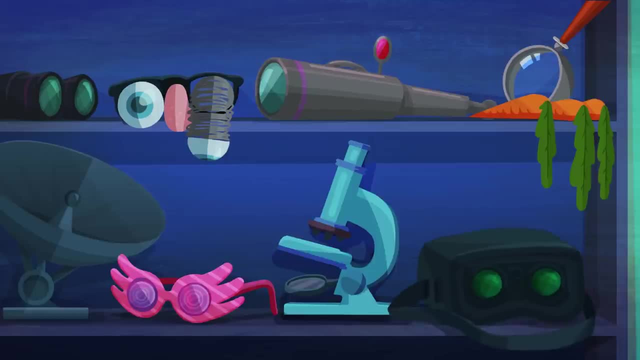 the dark. If we pass high-energy X-rays through them, the squirrels look very different. Humankind has invented lots of different instruments to show us what our eyes can see, Such as our Great Equatorial Telescope, which captures huge amounts of light and allows 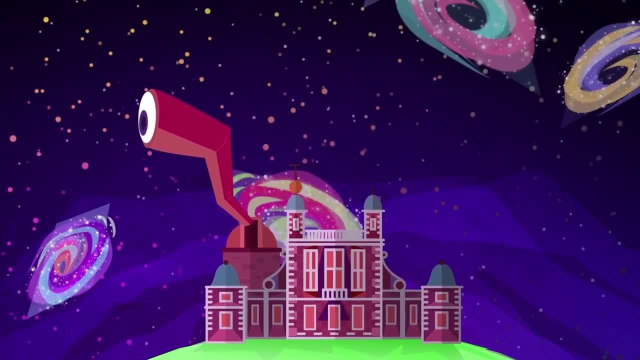 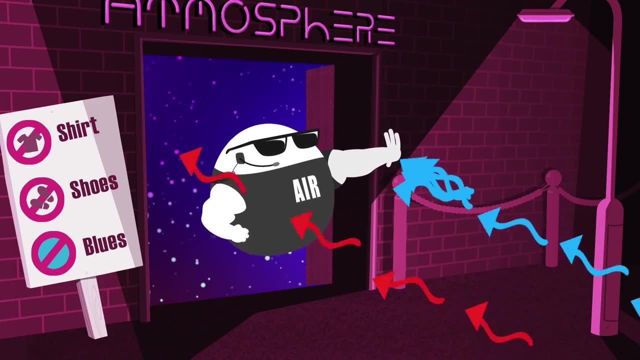 us to see objects that are tens of millions, of trillions of kilometres away. We can see matter interact with light and change it. The gases in the Earth's atmosphere scatter blue wavelengths of sunlight, giving us blue skies during the day and red skies at sunrise. 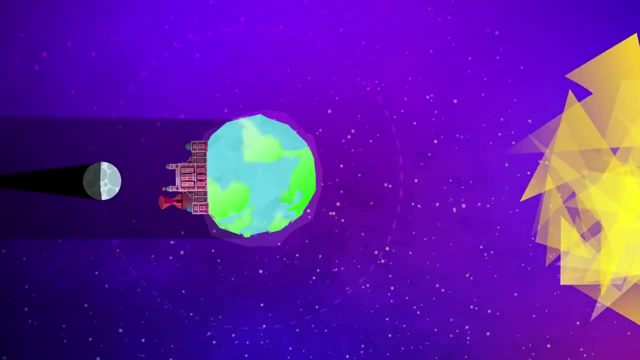 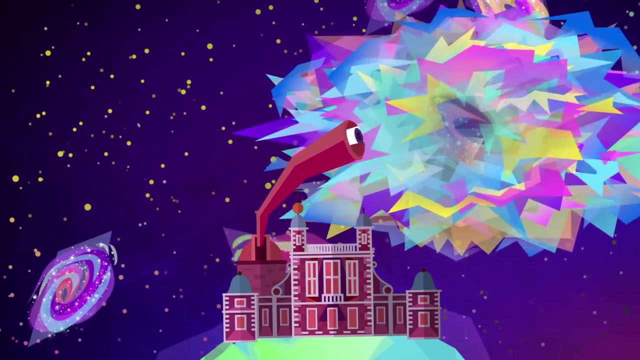 and sunset. We can watch sunlight reflect off planets and the moon During a lunar eclipse. red sunlight changes the light. The light changes the space and the sun changes the direction as it passes through the Earth's atmosphere and reaches the Moon. And although visible light from stars can be absorbed by dust in space we can detect. 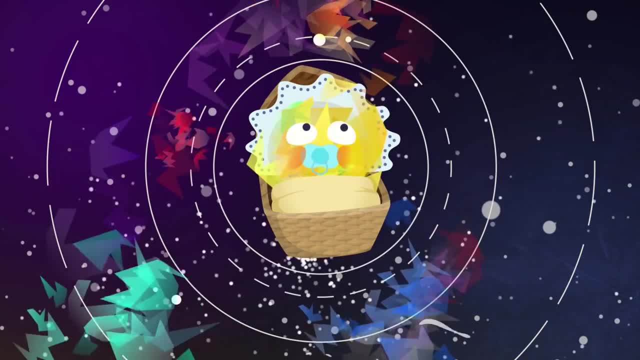 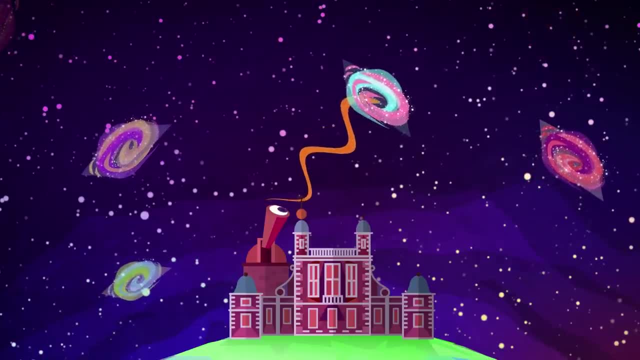 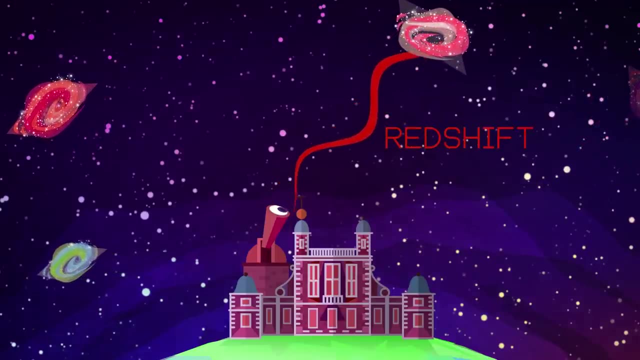 the infrared light which gets through to see baby stars hiding in nebulae. Light can even appear to stretch out. Since our universe is expanding and galaxies are moving away from each other, the light they emit is stretched to longer wavelengths. We call this redshift. 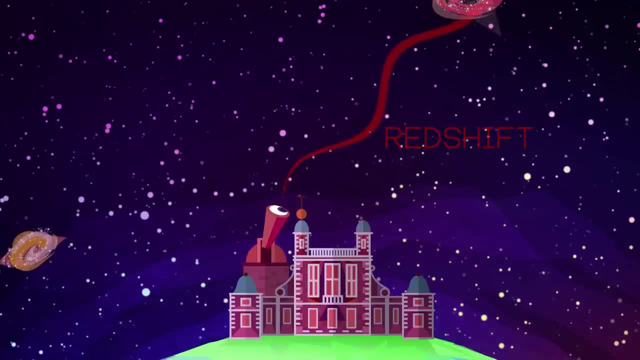 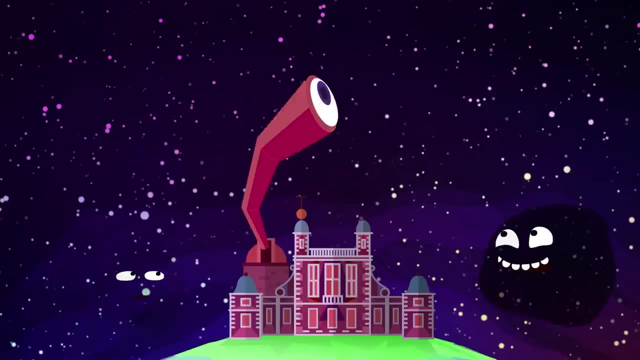 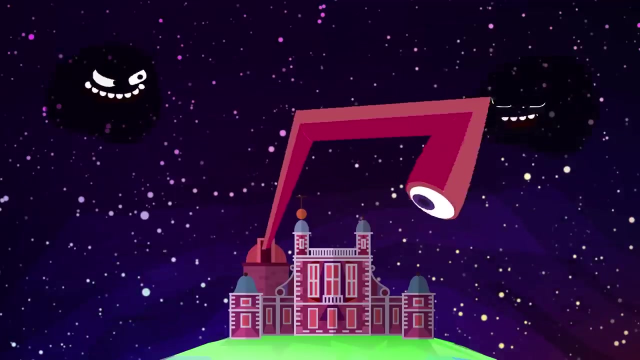 Some galaxies are so far away that their light has shifted and stretched from visible to infrared, so we can no longer see them. Stranger still, the universe has unknown amounts of dark matter and bizarre black holes, so even if we can detect all the different types of light, there are still some things in the